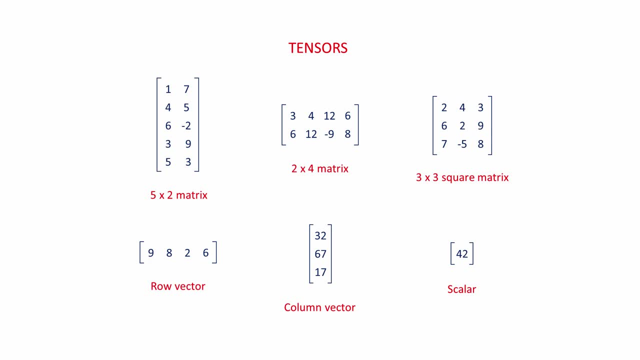 And a matrix is a tensor with an order And a matrix is a tensor with an order of 2.. A tensor can have any number of orders, but that is another story. So let's take a look at some simple operations that we can perform with matrices, starting with matrix addition. 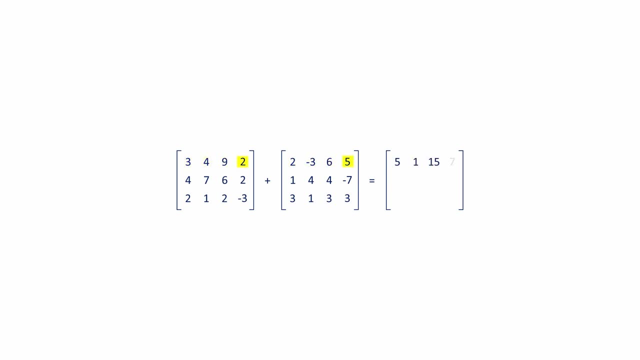 Well, this operation is rather simple. As long as the two matrices have the same number of rows and the same number of columns, you can add them together. It's just a matter of adding together corresponding values to generate a new matrix of the same size. 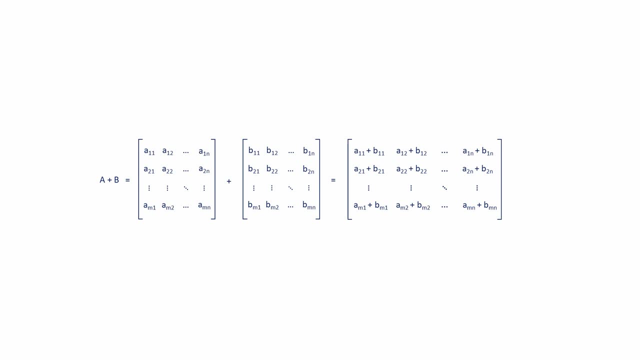 Algebraically, the addition operation can be described like this: You may come across this type of notation if you read around the subject. Each matrix is denoted by a capital letter. Every value in each matrix is denoted by the same letter in lower case. 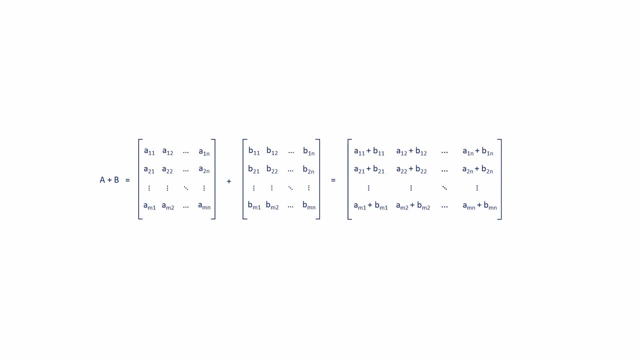 followed by its row number and then its column number. m is the total number of rows and n is the total number of columns. Of course, this kind of notation is really only useful if it helps you to understand the process. You can decide that for yourself. 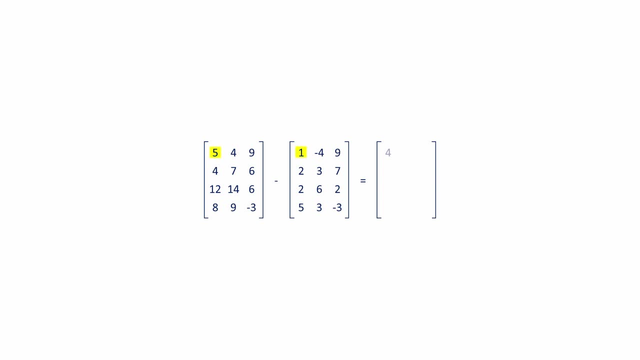 Matrix subtraction is just as trivial. As long as the two matrices are the same shape and size, we can subtract one from the other. In this example, a pair of 4x3 matrices result in a new 4x3 matrix. Algebraically, matrix subtraction can be described like this: 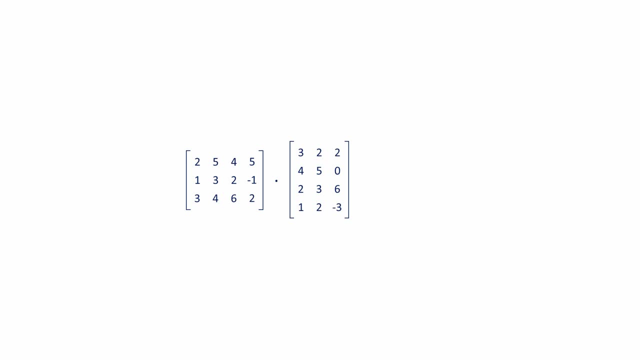 When it comes to multiplying matrices together, the most important thing to remember is that the number of rows in one matrix must match the number of columns in the other. In fact, if this isn't the case, you will probably lose your way if you attempt to do the calculation. 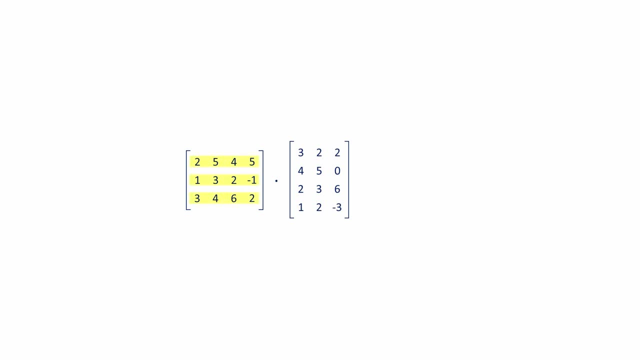 In this example, you can see that the first matrix has three rows and the second has three columns, so it is possible to multiply them together. The result, as you'll see in a moment, will be a 3x3 matrix. Notice that the symbol normally used to denote a multiplication operation is a dot. 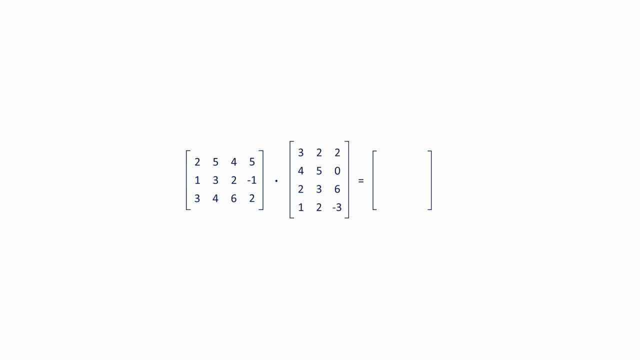 To multiply the matrices together. multiply each value in the first row of one matrix by its corresponding value in the first column of the other. Then sum up the products to get the first value of the new matrix Here. then 2x3 plus 5x4 plus 4x2 plus 5x1 gives us the value 39.. 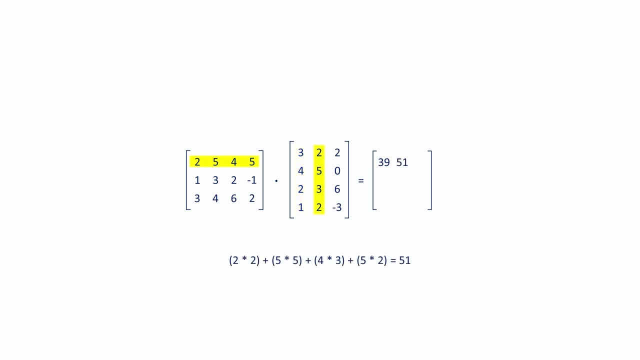 Next, multiply the values in the first row by corresponding values in the second column and sum up the products. Then multiply values in the first row by corresponding values in the third column and sum up the products. Next we want the sum of the products of corresponding values. 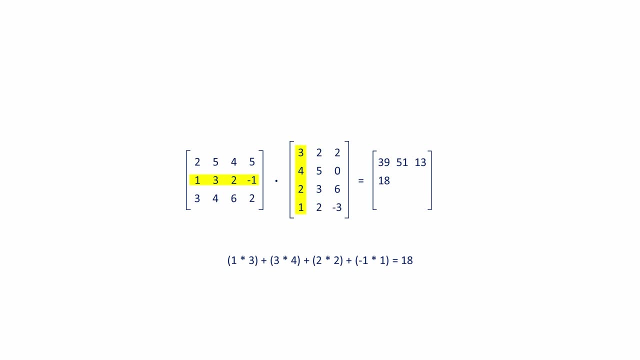 from the second row of the first matrix and the first column of the second matrix, Then the second row of the first matrix and the second column of the second matrix, The second row of the first matrix and the third column of the second matrix. 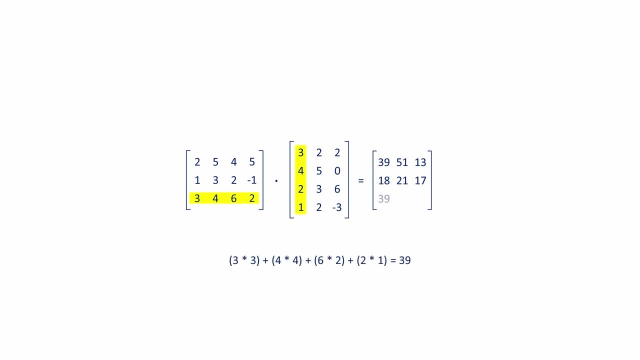 And then the third row of the first matrix and the first column of the second, The third row of the first matrix and the second column of the second matrix, And finally the third row of the first matrix and the third column of the other. 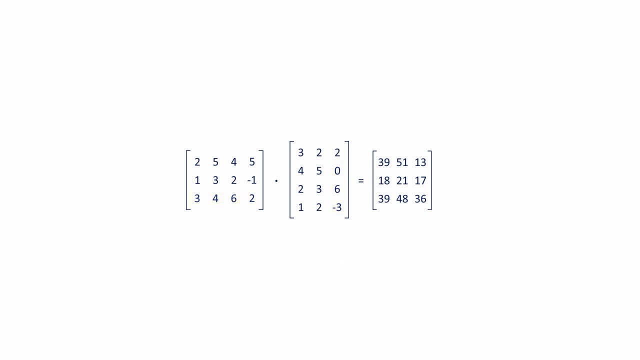 As you can see, calculating the product of a pair of matrices is a slightly more complicated process than addition or subtraction, but you'll get the hang of it with a little practice. I suggest you give yourself a few examples to do with simple numbers like these, so you can focus on the method. 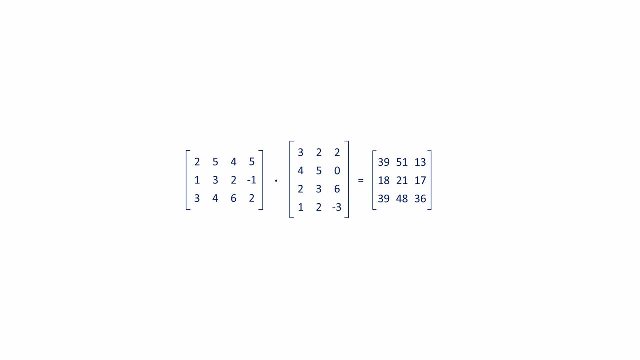 Perhaps try a pair of larger matrices. You could even try multiplying a pair of square matrices together. You can check your own solutions online. There are plenty of free matrix calculators available that will let you do this easily. By the way, matrix multiplication: 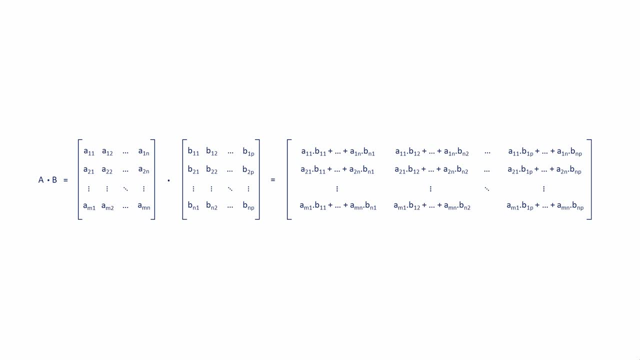 can be described algebraically like this: Notice from the subscripts that the first matrix is being referred to as an m by n matrix and the second as an n by p matrix. This emphasises the rule that m in the first matrix must match n in the second.